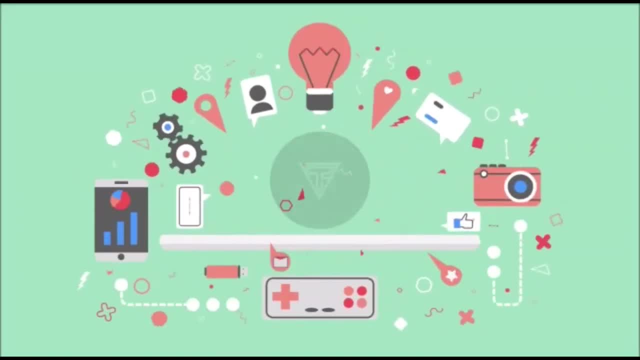 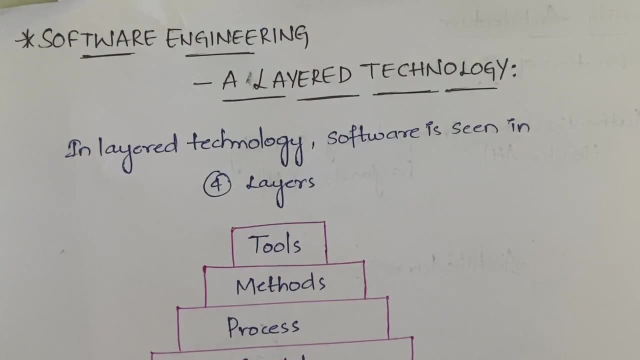 Hello everyone, welcome back to my YouTube channel, Rubble Free. In this video, I'm going to explain you about software engineering, a layer technology. in the subject of software engineering, That is, we are going to see software in terms of four layers. Okay, and 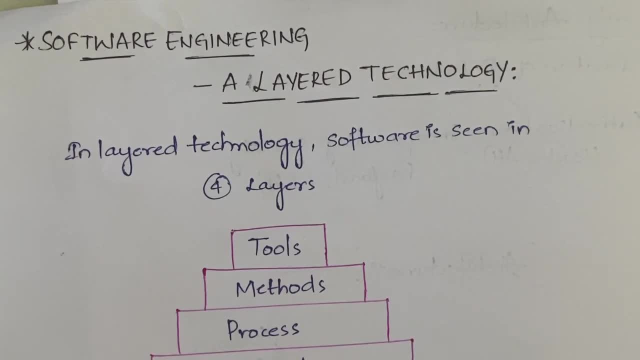 what are those four layers? What does each layer means? Everything we will be understanding in this video, Okay. so let's get started, And before that I have already sorry- I have also started a new channel with study abroad content, If you are interested, you. 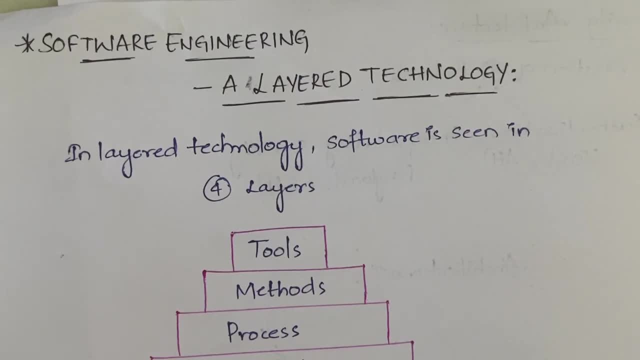 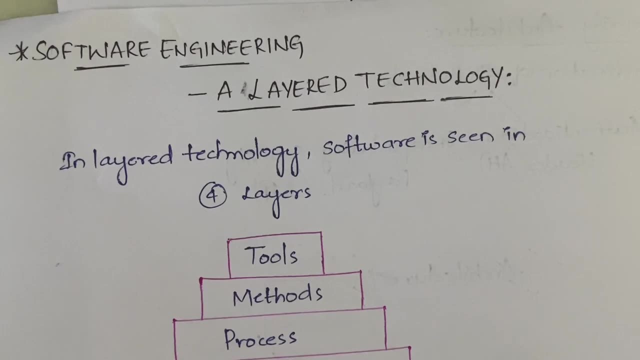 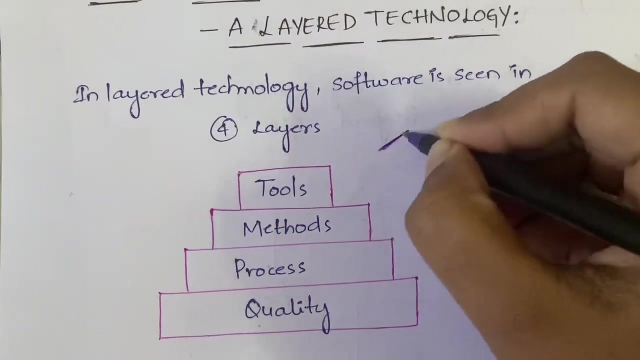 can have a look at that channel And let's get into the video now. So basically, a layer technology. in the layer technology we are seeing software as a four layers form And in that four layers we have tools, methods, process, quality. So you can remember it as: 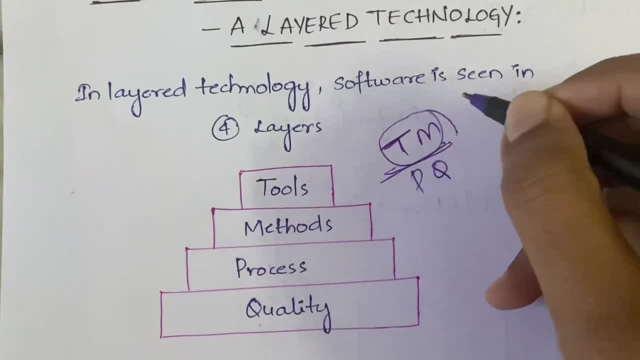 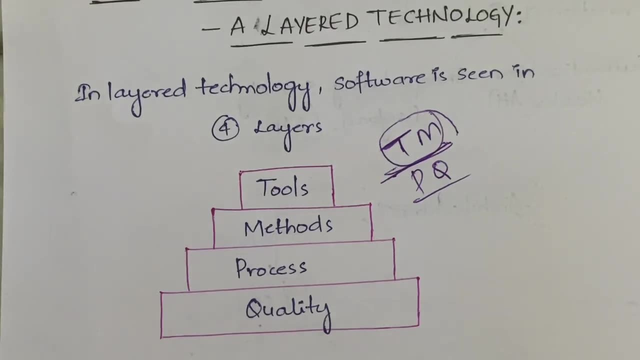 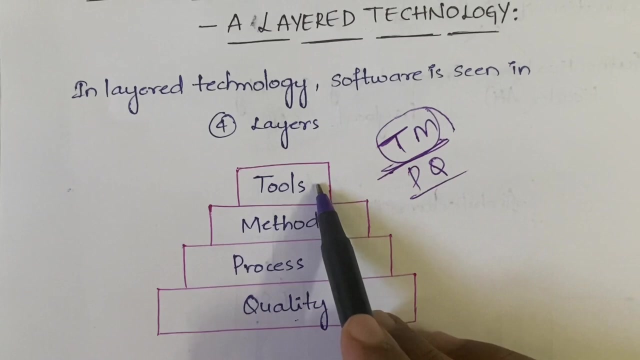 Q, So TM. let us remember it as time management or something like that. So TM and PQ. you know simultaneous alphabets, like that. you can remember Tools, methods, process, quality, Okay, so in that, first is tools. So tools are nothing but they will provide. okay, but like instead. 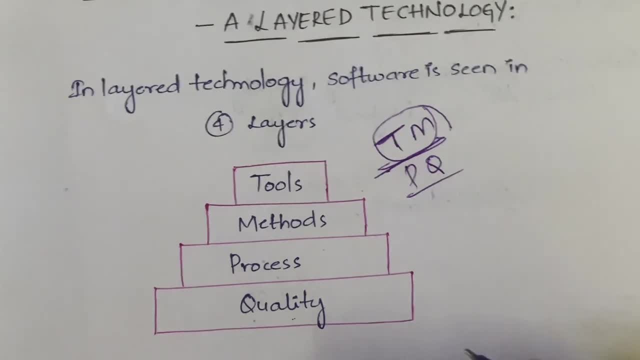 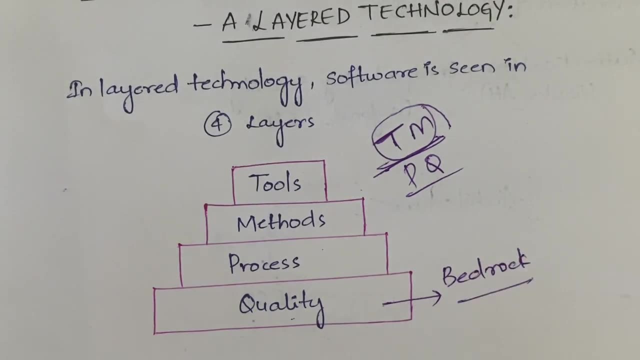 of going from tools to quality. we will go from quality to tools. Quality is a bedrock. It is a bedrock that supports a system, SC. So what do you mean by bedrock When you are constructing a house? we will be, will be. 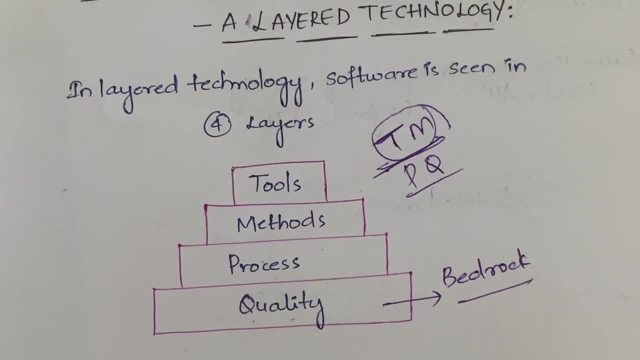 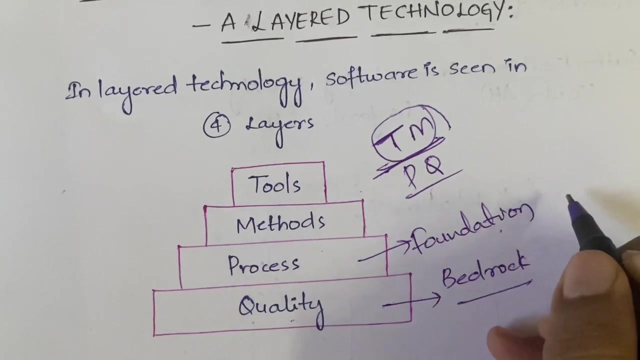 saying bed, bedrock, that is a support, A basic foundation kind of thing. we can say, Okay, It is a bedrock that will support the software engineering Got it Next. process, Process as a foundation, Process is a foundation for SC. Quality is a bedrock that will provide. 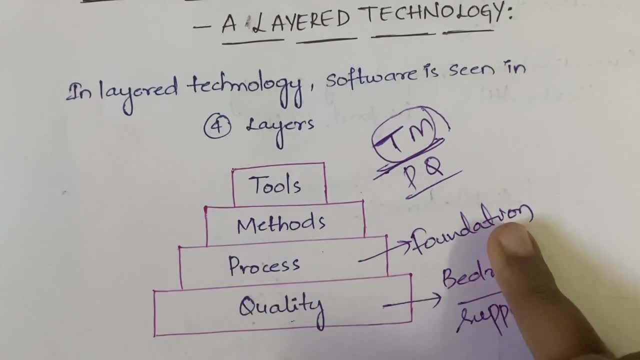 support to the software engineering And process is a foundation for software engineering. Process is a foundation formaking code, software engineering and methods. methods will provide you technical how to's for building a software that is for each and everything. how to do this, how to do if a software is having some.